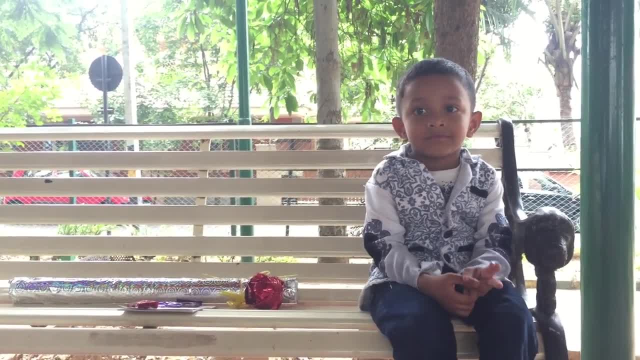 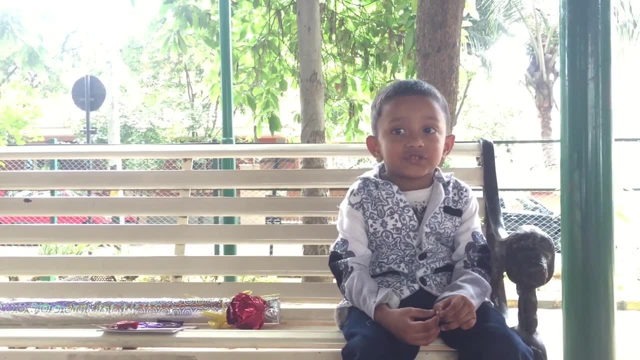 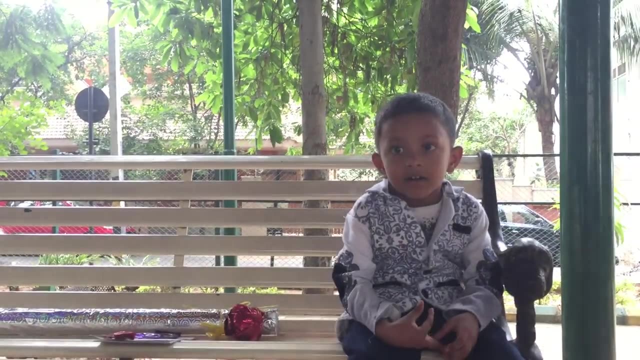 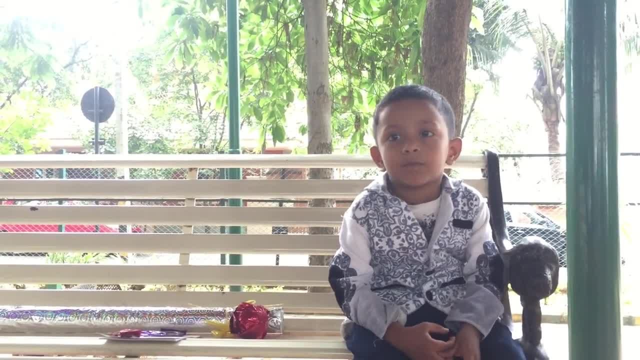 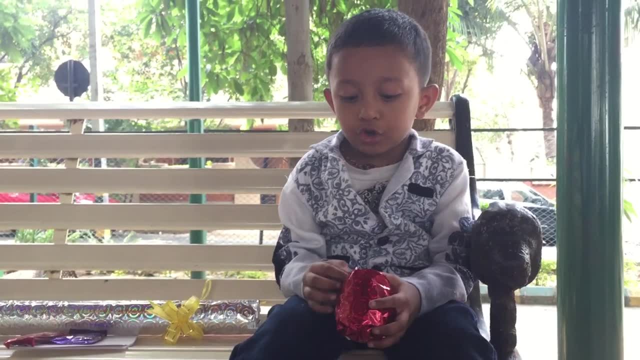 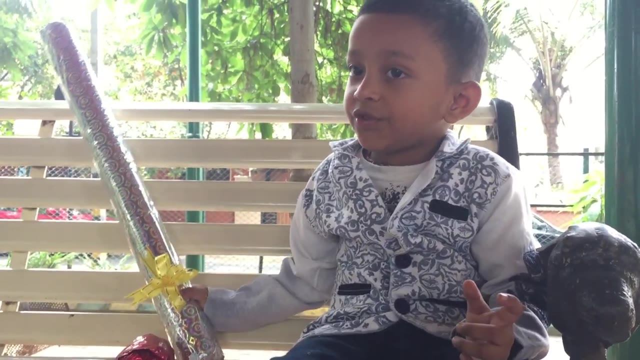 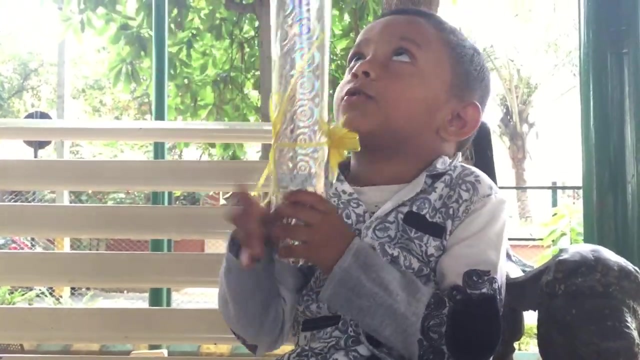 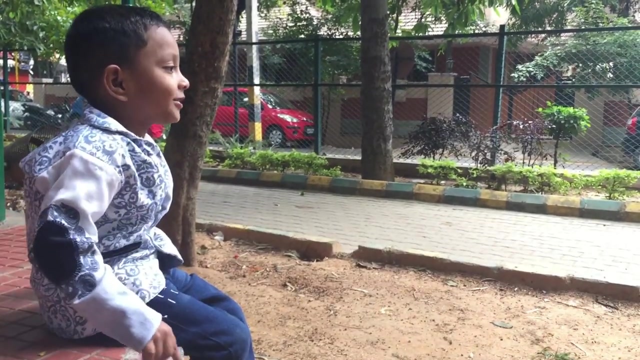 Okay, and which planet do you like? Black European Space, Space, Right, Okay, what are your favorites? So next time I will tell you what are the planets in our solar system, Which are the planets which have rings: Earth, Venus, Mars and Jupiter. 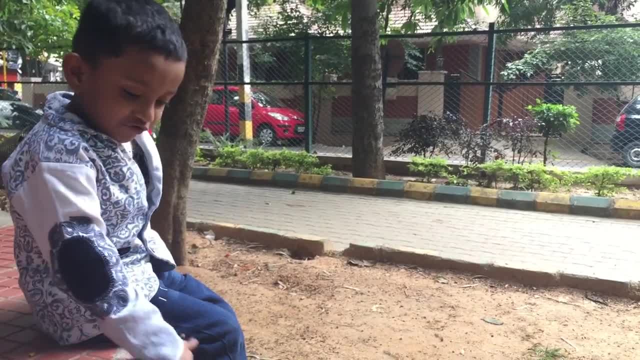 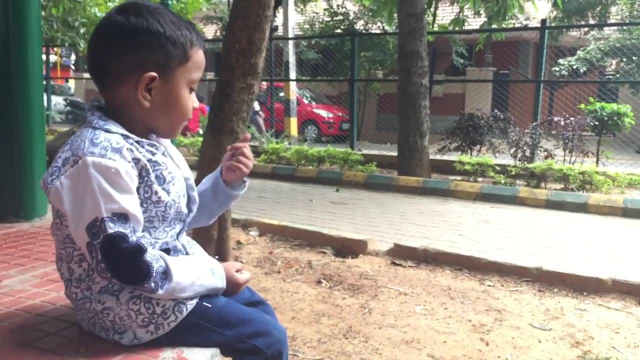 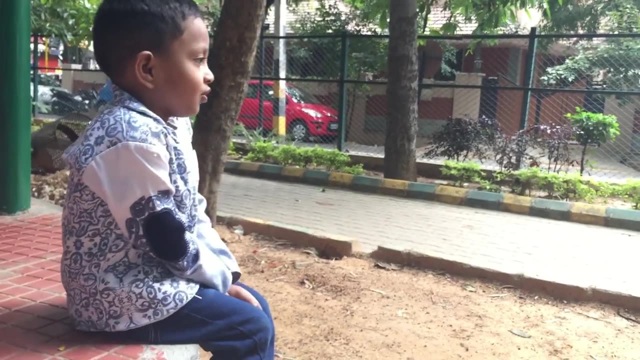 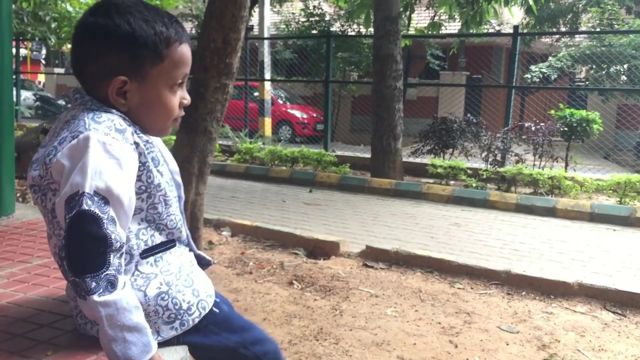 Which is the hottest planet? Mercury and Venus, Which are the dwarf planets? Huh, Which are the dwarf planets? Sirius, Mercury, Pluto and Io? Ok, very good, So he said four dwarf planets. Which is the closest planet to the Earth? 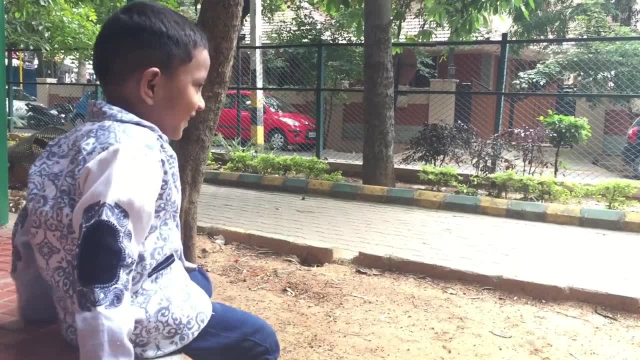 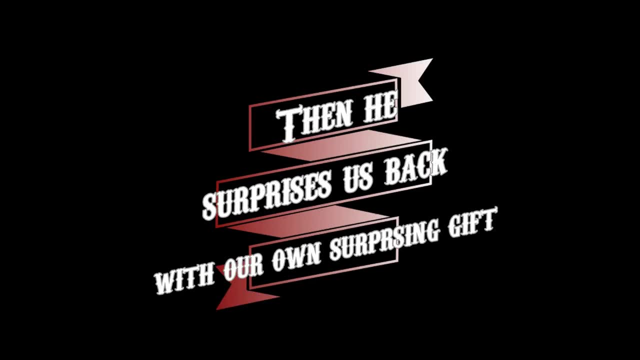 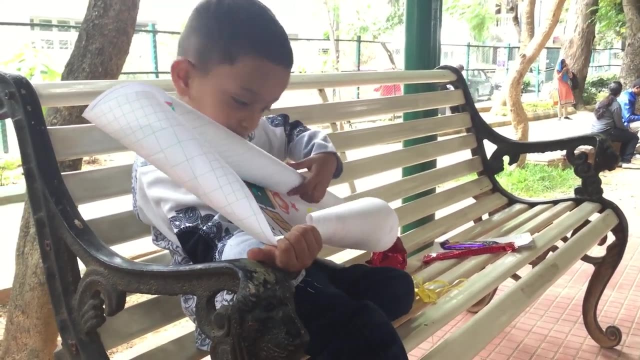 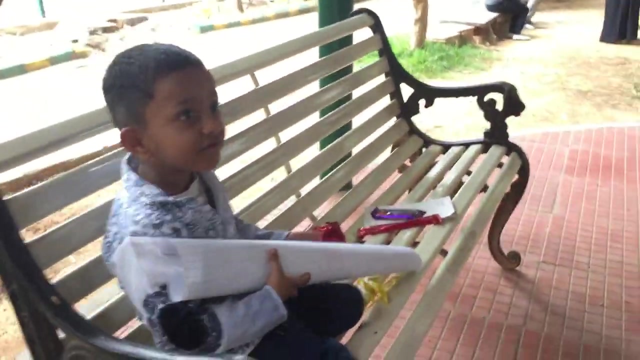 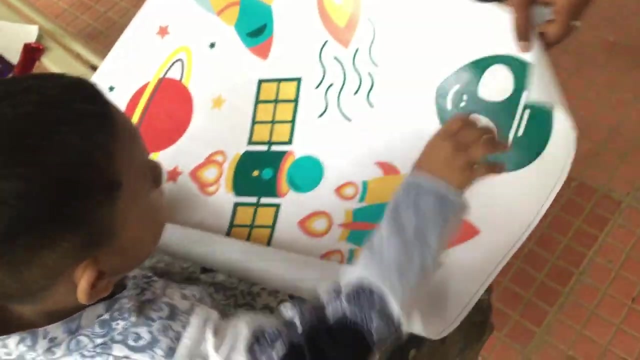 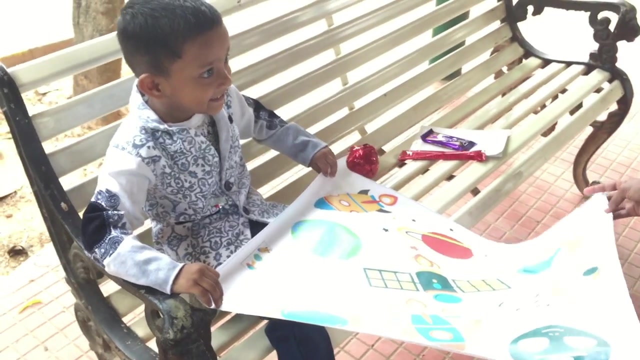 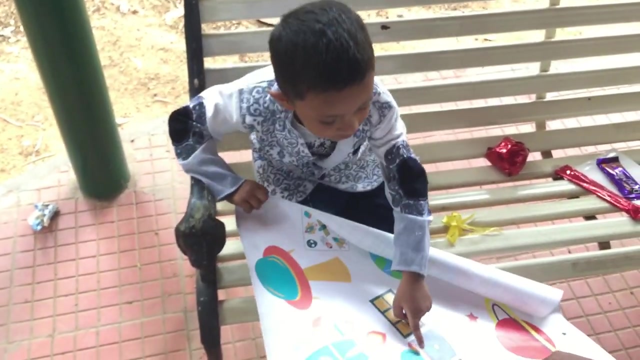 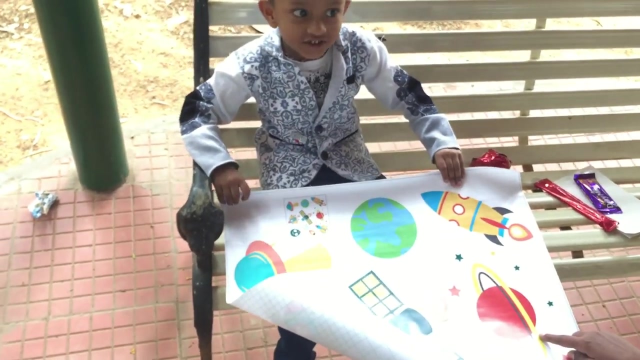 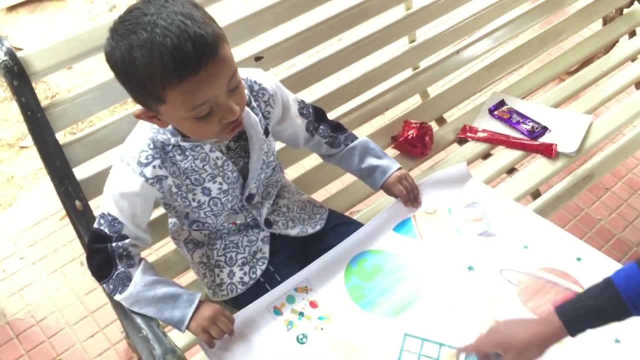 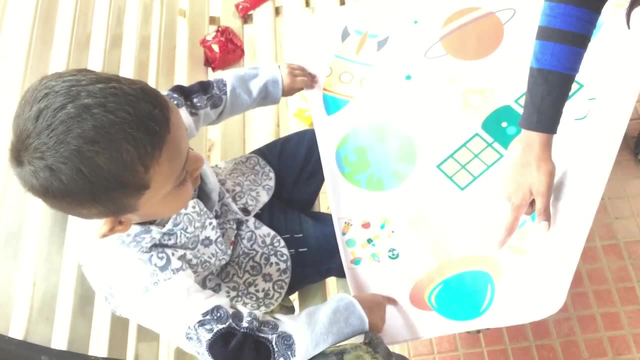 Saturn, Very good. And what is this Aliens? Who is this then, Aliens? This is alien. right, Very good. And what is this Rocket? Rocket, Did you like it? Yeah, Wasn't he amazing.